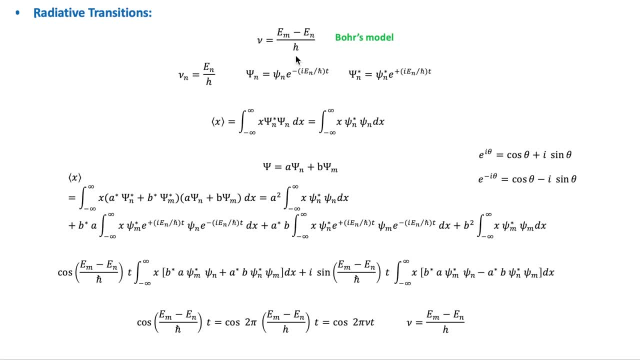 So we will now show that this equation arises naturally in quantum mechanics. So suppose that a system is in a certain quantum state, n. Then the time-dependent wave function, psi n, is equal to psi n, e to the power of minus i en over h bar t. 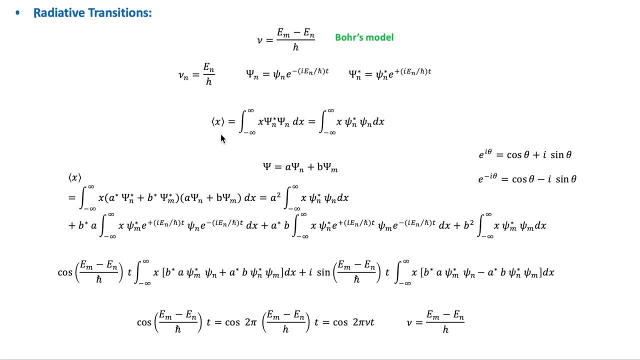 And the expectation value of the position of this electron Is given by this equation, Which is equal to the integration of x times the complex conjugate of psi, n, dx. And this integration here is a constant in time, because these two functions are functions of position only. 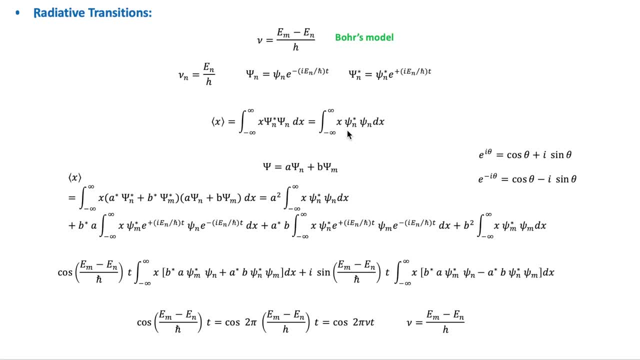 And so this means that the electron in this case does not oscillate and so no radiation occurs. So this shows that quantum mechanics predicts that a system in a specific quantum state n does not radiate, And this is known from before and observed in experiment. 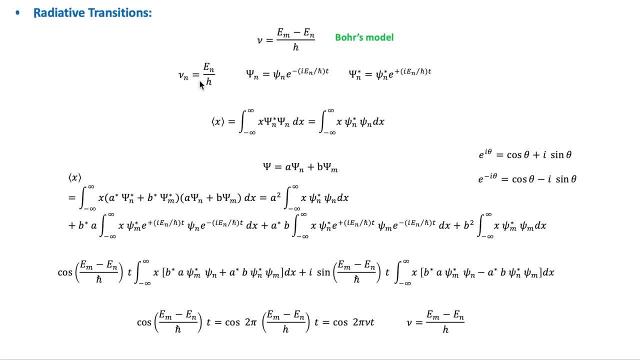 So now let's consider an electron that shifts from one energy state to the other. This happens, for example, when a system is in its ground state n and then is excited through a beam of radiation Or through a collision with another particle. 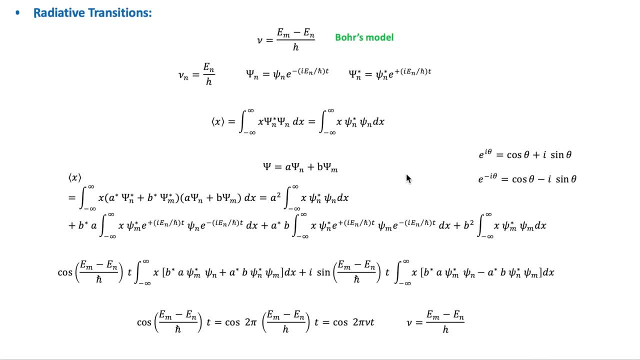 So it is excited to another quantum state, m, And then in that case the system will emit radiation as it transitions from the excited state em to the ground state en, And during the time of transition the electron can exist in both states n and m. 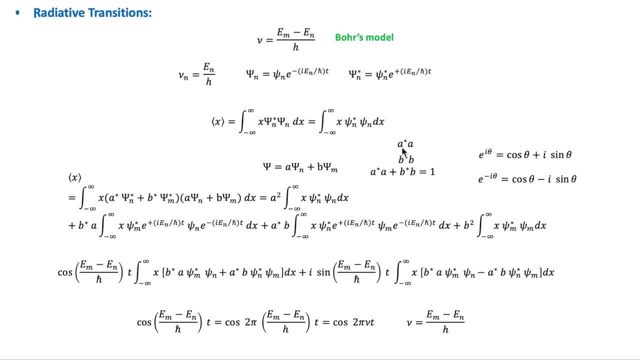 So a conjugate a is the probability that the electron exists in the state n, And b conjugate b is the probability that it exists in the state m, And the sum of these two is equal to 1.. So initially, when the electron is in the ground state, a is equal to 1 and b is equal to 0. 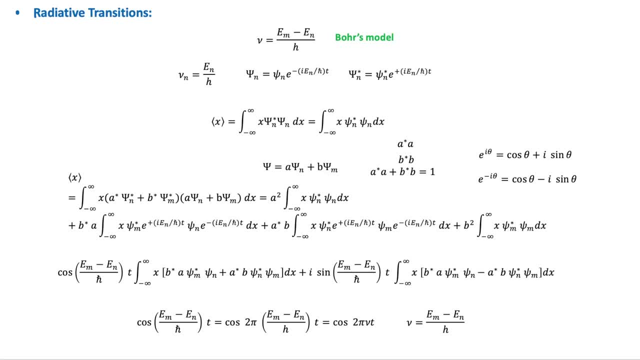 And when the electron is in the excited state m, then b is equal to 1 and a is equal to 0.. And when it goes back to the ground state, then a is equal to 1 again and b is equal to 0.. 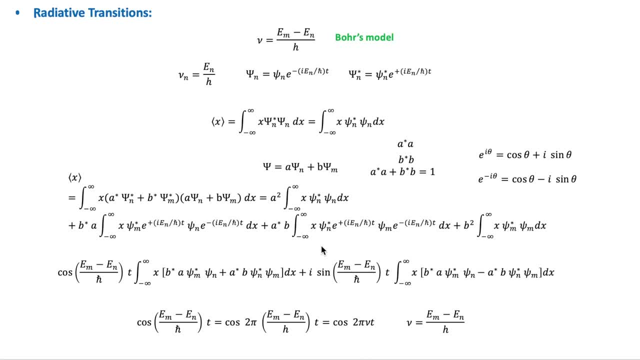 So when the electron is in either of the quantum state n or m, we know from this equation that it will not oscillate and no radiation occurs. But during the time of transition from m to n, which is when both a and b are in the excited state m, 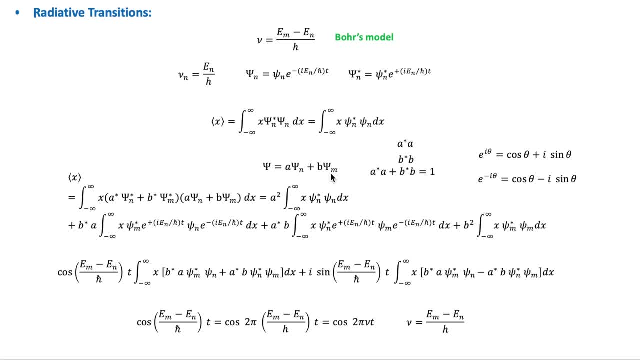 which is when both a and b are in the excited state m, which is when both a and b are in the excited state. m and b are not equal to 0,, then the electron will oscillate and radiation occurs, So the system will emit electromagnetic waves. 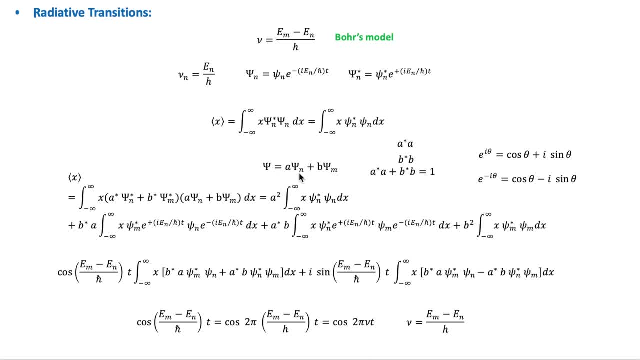 So, using this wave function during the time of transition for the electron, the expectation value during this time is given by this equation. So we know from this equation that the first, the first and last integrals here do not vary with time. okay, 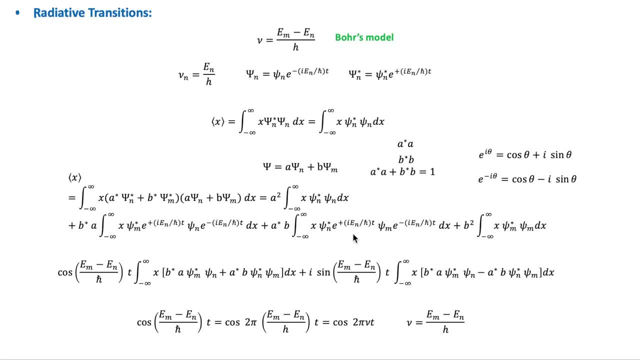 And now we have these two integrals here which vary with time And we, using these two expressions for the exponential, we can write these two terms this way: okay, And this is the imaginary part and this is the real part which, as you can see, does vary with time. okay, 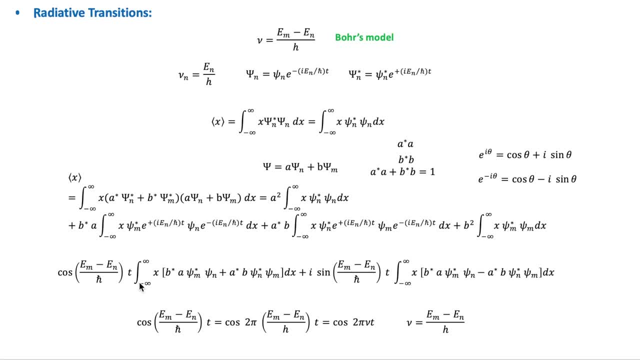 And so this shows that the electron's position oscillates simultaneously with the frequency em minus en over h, because this is equal to 2 pi em minus en over h T, and this is the frequency of oscillation. So this shows that if the electron is either in the quantum state n 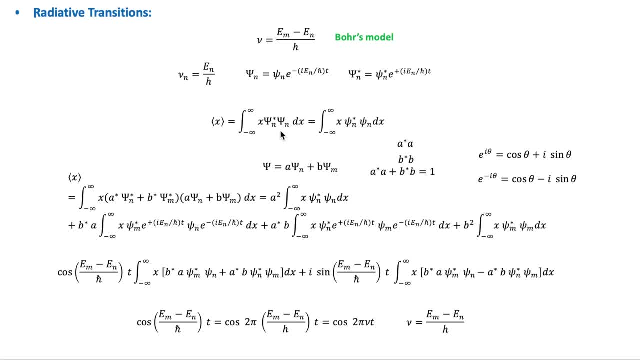 or m, then from this equation it shows that the expectation value for nc is equal to m In the quantum state. we will get m again, which is Сов by m right. So this shows that if the electron is either in the quantum state n. 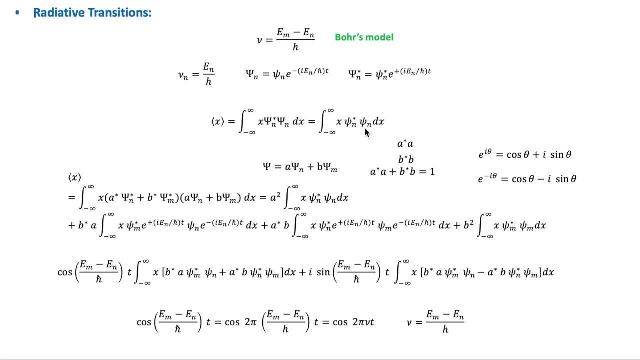 or m, then from this equation it shows that value of the electron's position is constant, and so the electron does not oscillate and will not emit electromagnetic radiation. but when the electron undergoes a transition between the two states n and m, then the expectation value or its position oscillates with a frequency. 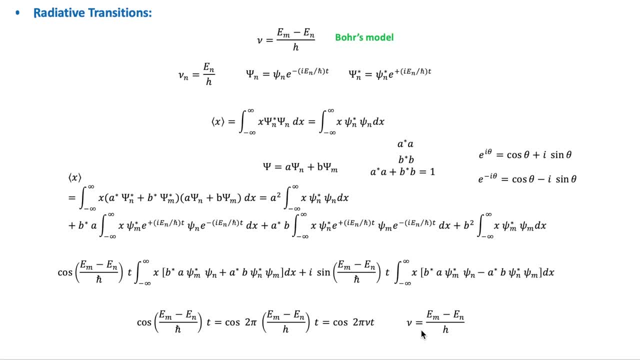 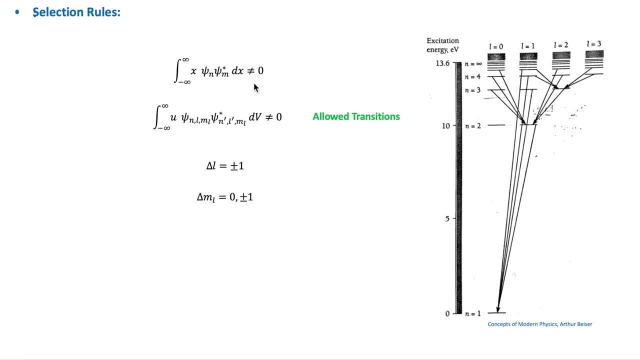 mu. okay, and so the electron does oscillate like an electric dipole and radiates electromagnetic waves of frequency mu equal to em minus en over h, and this result is the same as the one postulated by Bohr. so, as we have seen, this integral is related to the electron oscillating and 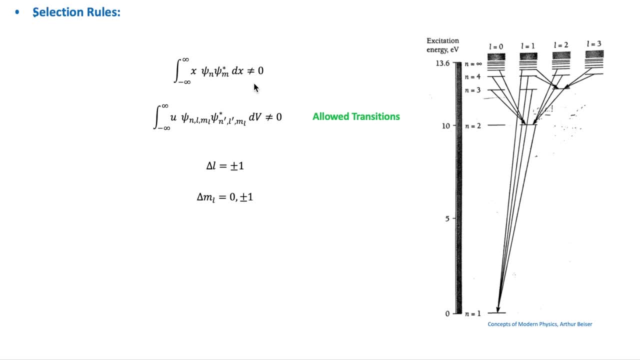 radiating electromagnetic waves as a result. okay, you um. so the general condition necessary for for an atom in an excited state to radiate is that this integral is not equal to zero. so transitions for which this integral has a finite value is known as allowed transitions, and those for which this integral is zero are forbidden. 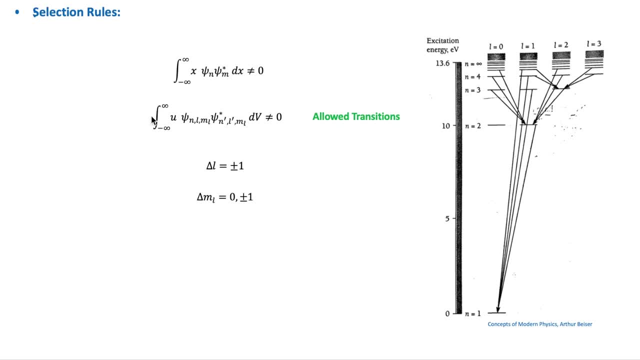 transitions, okay, and in the case of the hydrogen atom, three quantum numbers are needed to be able to radiate the energy of the electron, so the general condition necessary for allième. rewards are then needed to specify the initial and final states, which are n, l, m, l. 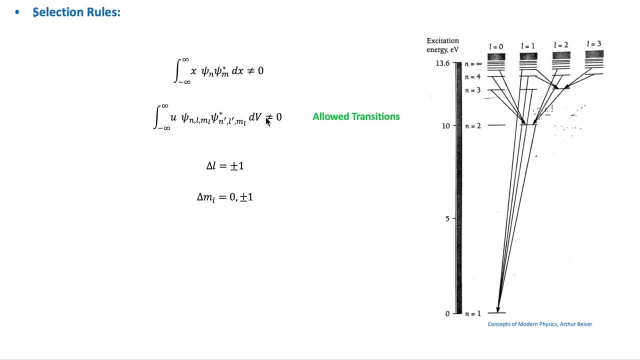 so the allowed transitions are the ones where this integral is not equal to 0. so the integral here is over all space, and if u is equal to x, then the radiation would be the one corresponding to a dipole oscillating along the x axis. okay, and if it's y, then it's a dipole along the x axis, and if it's for this, поэтому, 지�� radiator" along the x axis- okay, and if it's y, then it's dire龍的到 x 시간. a dipole along the x axis- okay, and if it's y, it's a dipole along the x restaurant, that is, the hyperbolic cierti. 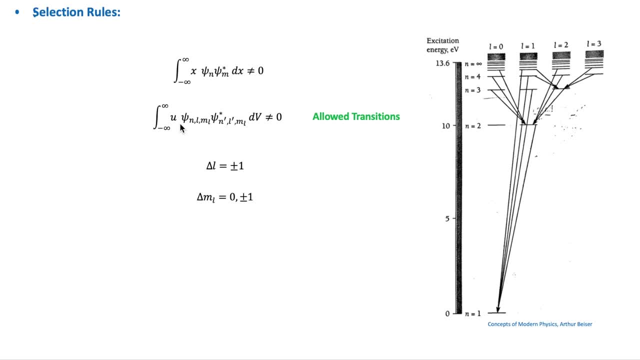 then it's a dipole along the y-axis, and so on. okay, so because the wave functions psi, n, l, ml for the hydrogen atom are known functions, then it is possible to evaluate this integral for u either equal to x, y or z for any pair of states that differ in one or more. 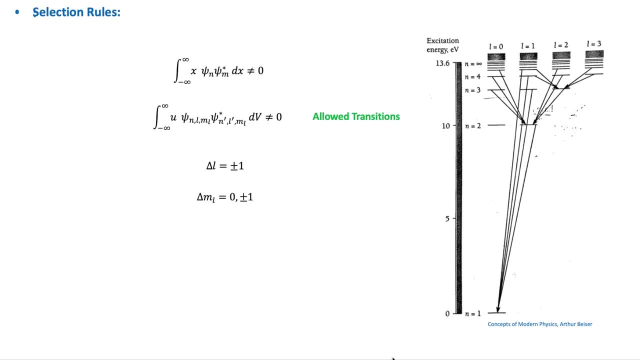 quantum number. so after these calculations were done, it was found that allowed transitions between different states of different principal quantum number n can occur if the orbital quantum number l changes by either plus or minus one and if the magnetic quantum number ml either does not change, so that changes zero, or it changes by plus or minus one. 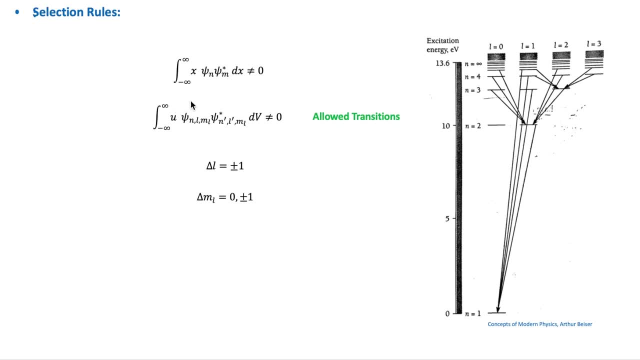 so this shows how selection rules arise naturally in quantum mechanics due to the wave nature of the electron, and how not any transition is allowed, but only those transitions with these selection rules. okay, and note here that the change in the principal quantum number is not restricted in any transition. 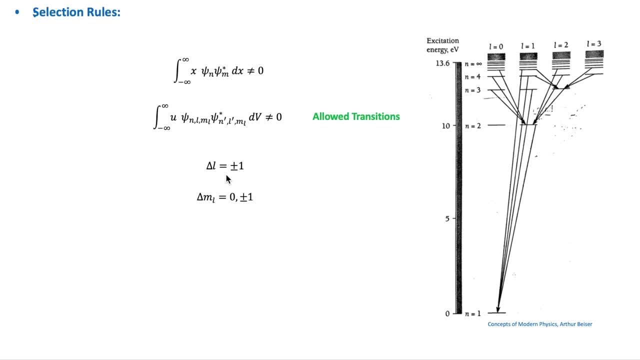 and note here that from the conservation of angular momentum this selection rule means that if an atom makes a transition between two states and radiates, then the emitted photon will carry the angular momentum of plus or minus h bar. so the angular momentum in which the photon carries is equal to the difference between the 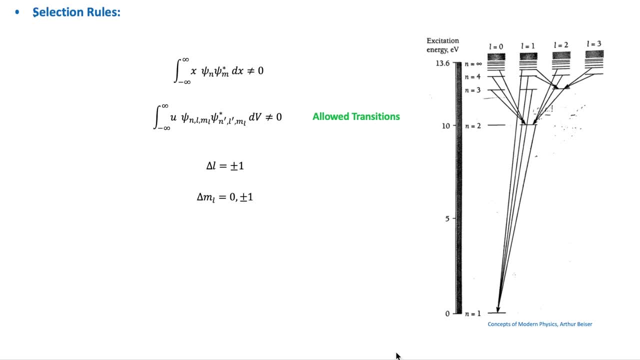 angular momentum of the atom's initial and final states and in the classical theory of electromagnetic radiation, a photon with angular momentum of plus or minus h bar corresponds to a left or right circularly polarized electromagnetic wave respectively. so this figure shows the energy diagram in a hydrogen atom and it shows the allowed transitions. 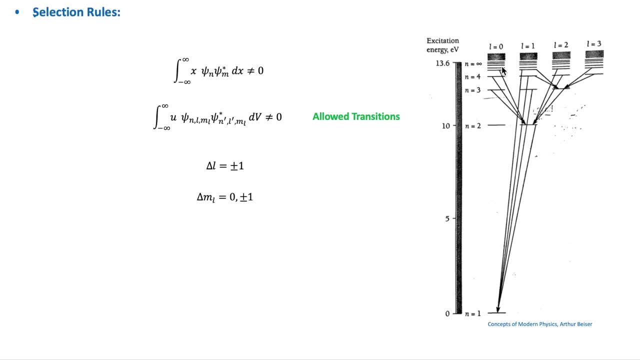 and, as you can see, only those where l differs by plus or minus 1 can occur. so now let's consideribiq as shown here, for example, hydrogen atoms being transcribed by plus or minus one maQ, and that's only those where the cocoa only differs by plus or minus one maQ. 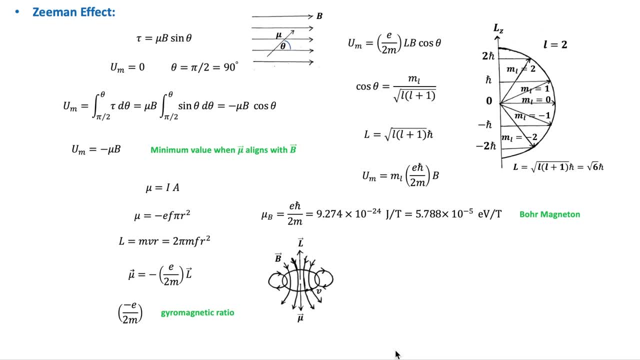 so now let's consider here for a Video, video at the big data square operation. so now let's consider what happens to an atom when placed in a magnetic field. so in the previous videos of electromagnetism we have seen that the magnitude of the torque tau. 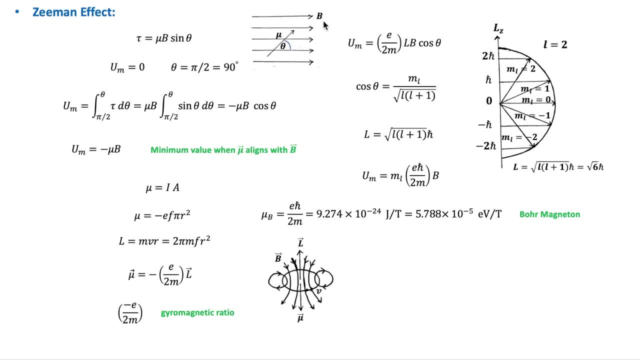 on a magnetic dipole, mu placed in a magnetic field of flux, density b is equal to mu b sine theta, and theta is the angle between the two vectors, mu and b. okay, and so from this you can see that the torque has a maximum value when the dipole moment is perpendicular to the field and the angle. 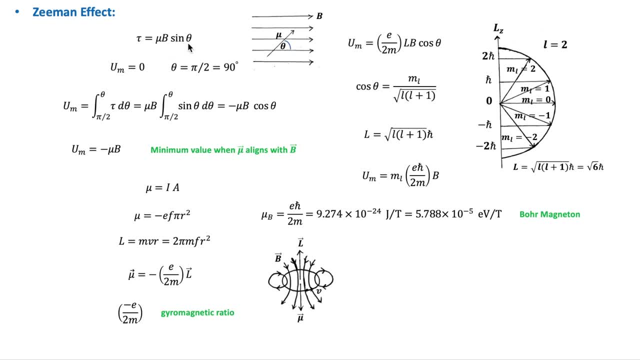 is 90 degrees and the torque is equal to zero when the dipole is either parallel or anti-parallel to b. so now let's set the reference configuration where the potential energy of the system is zero. okay, because, as we have seen in mechanics videos, only the changes in the potential energy are meaningful. 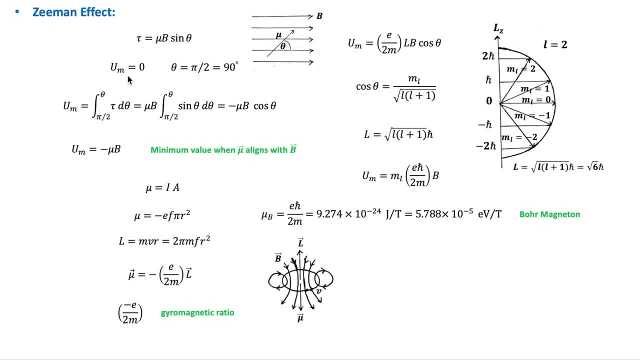 or observed. so the choice of the reference configuration is arbitrary. so what is meaningful is delta u, not u. okay, so let's assume now that the magnetic potential energy is zero when theta is equal to pi over two, so when the magnetic moment is perpendicular to the field b. 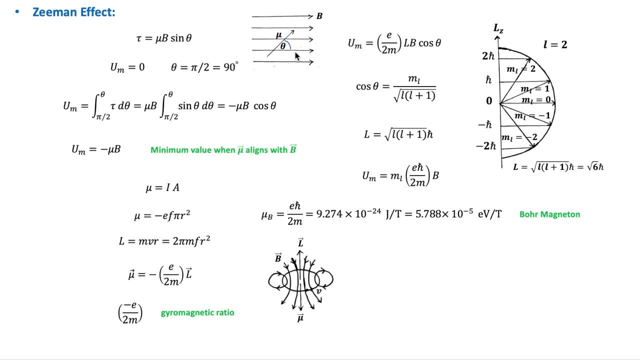 so the potential energy at any other angle is equal to the amount of external work needed to rotate the dipole from theta naught equal to pi over 2 to theta. so the work done is the integration of tau d theta from pi over 2 to theta. 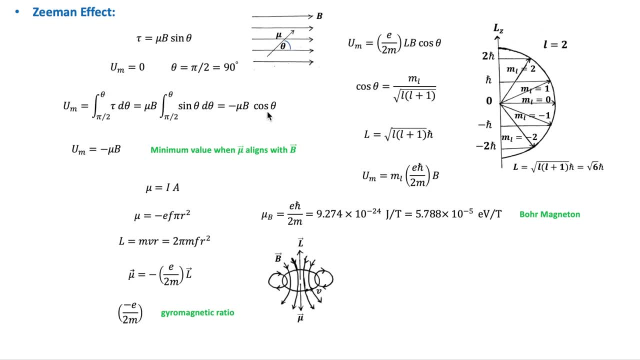 equal to minus mu, b cosine theta. okay, so this shows that when the magnetic moment mu is in the same direction of b, so when mu aligns with the external magnetic field b, then the magnetic potential energy will have a minimum value, and this is why a magnetic dipole. 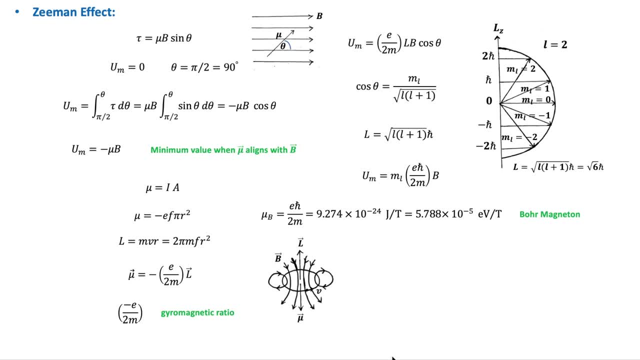 tends to align itself with an external magnetic field, because the potential energy of the system would then be minimum for that configuration. so now let's see how the magnetic dipole moment of the electron relates to its angular momentum. so we know that the magnetic moment of a current loop is equal to ia, where i is the current and a. 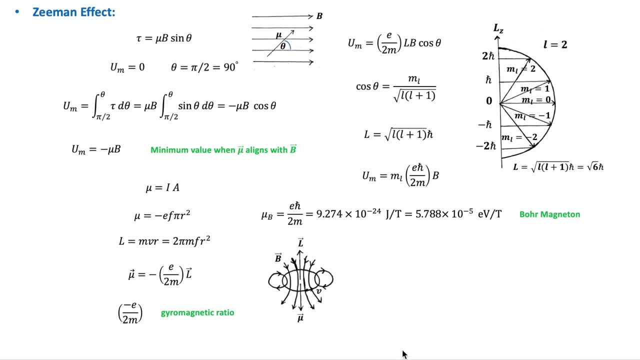 is the area of the loop, and so an electron that makes f revolutions per second in a circular orbit produces a current of minus ef, and so mu is equal to minus ef. pi r square, and the angular momentum of the electron is mvr, and we know that v, the linear speed of the electron is equal to 2 pi fr, so the so l is equal. 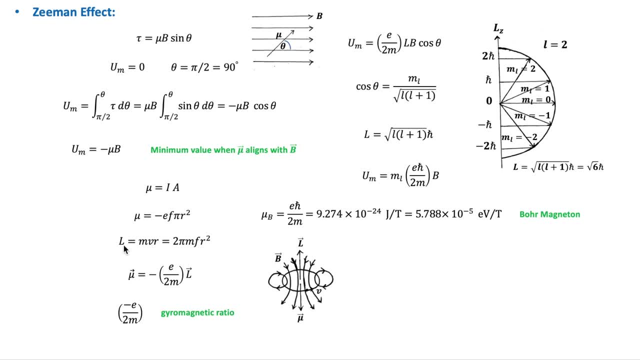 to 2 pi m of r square, and so the magnetic competed by the electron is equal to mega pi m l if i, το wr rez sufferingante moment vector is equal to minus E over 2m L, and this ratio is known as the gyromagnetic ratio, and the minus sign indicates that mu is in opposite. 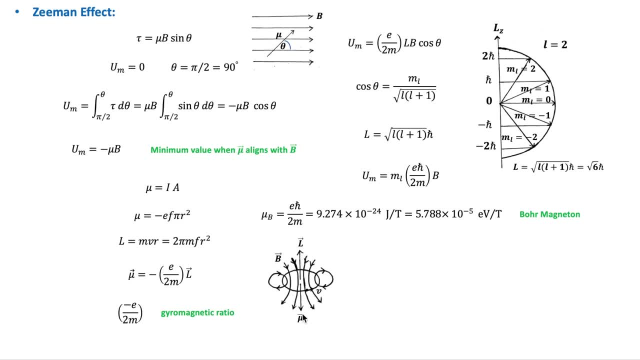 direction to L, and this is because the electron has a negative charge. so now, if we substitute this here, we get the magnetic potential energy of an atom in a magnetic field. so it depends on both theta and B, and from the previous video of the hydrogen atom we know that the angle between the total angular momentum 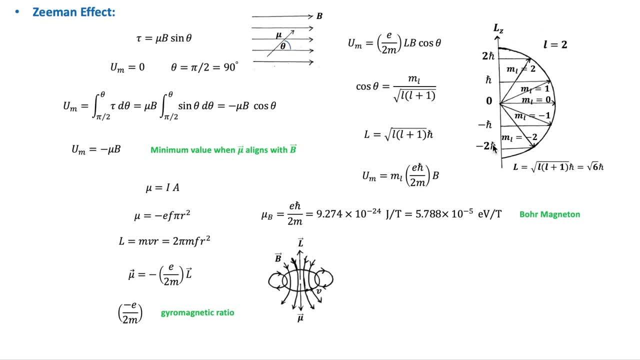 vector L. this vector and the z-axis can only have these specific values. okay, so these are the possible orientations. in the case of L equal to so, there are two L plus one L and two L minus one L. so these are the possible orientations. in the case of L equal to so, there are two L plus one. 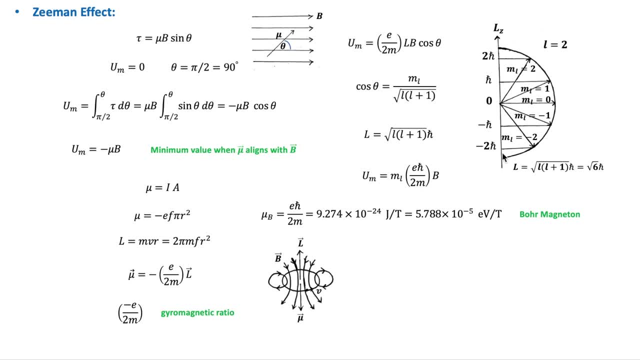 possible orientations in an external magnetic field, which is in this case five orientations, and the magnitude of the vector. the angular momentum vector L is equal to square root of six H bar. okay, so we substitute these results from quantum mechanics for the quantization of the direction of the angular momentum. 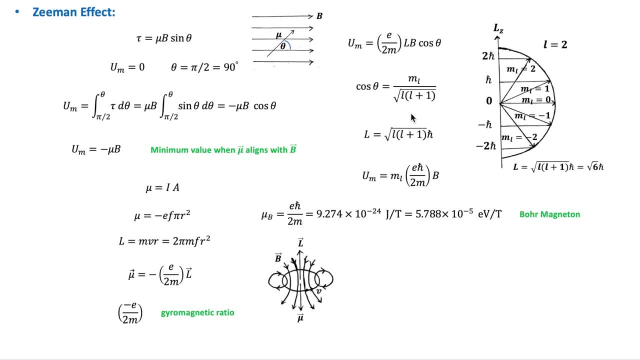 of the electron and the quantization of its magnitude into this expression of the potential energy of a magnetic dipole in an external magnetic field. and we get this expression and this quantity here is known as the Bohr magneto. so when an atom is placed in an external magnetic 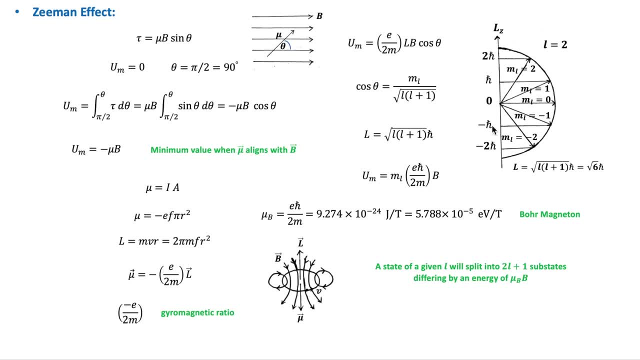 field, let's say along the z-axis, then the energy of a particular state will not only depend on the principal quantum number n, but also on the magnetic quantum number ML, because a certain state of a particular orbital quantum number L will break into or split into two L plus one sub states. okay, differing. 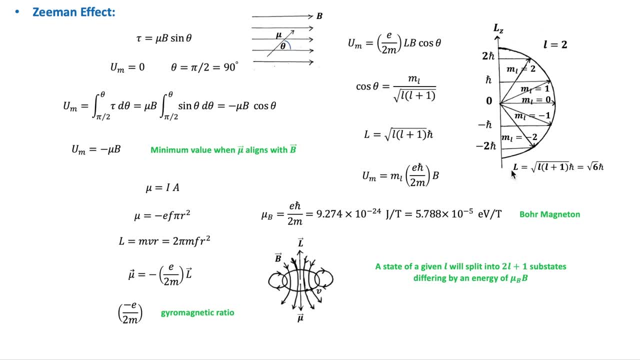 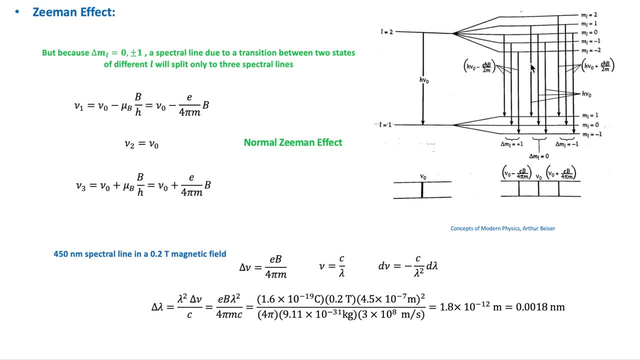 in energy by mu, B, B. so these are the are different energy states as a result of placing the atom in an external magnetic field. so these are the are different energy states as a result of placing the atom in an external magnetic field, but because the changes in ML are restricted to. 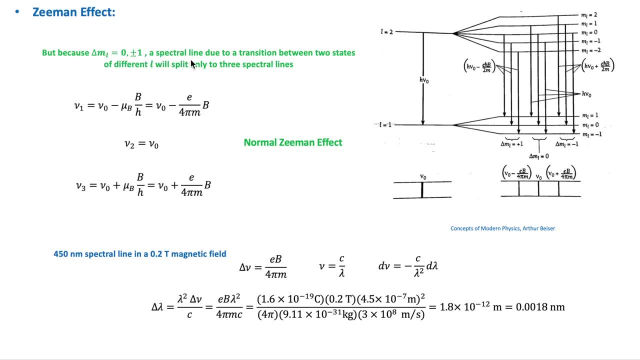 either 0 plus or minus 1, then a spectral line due to a transition between two states of different L will split only to three spectral lines. so this spectral line of a certain transition will now split to three spectral lines when the atom is placed in an external magnetic field. 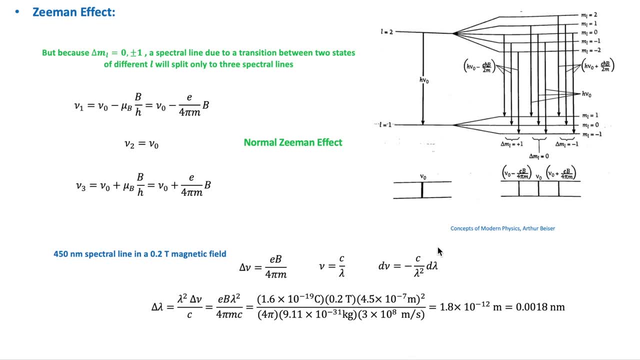 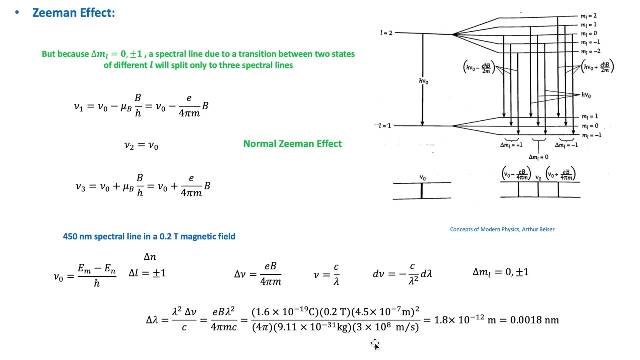 and this is known as the normal Zeeman effect. so mu naught will split into mu 1, equal to this value, and mu naught, the original frequency, and mu 3, okay, equal to this value. so as an example, consider an atom of a certain element that when 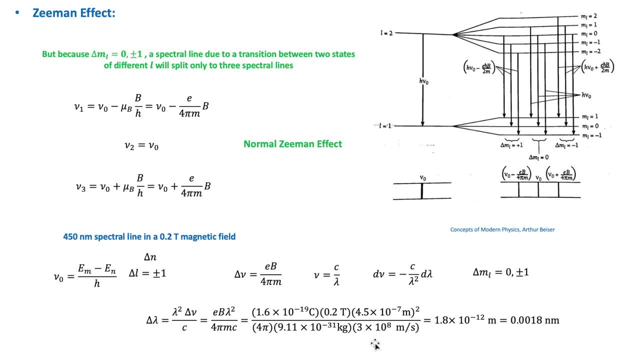 excited and when it drops back to the initial state it gives a spectral line of a wavelength of 450 nanometers. so this means that an electron in that atom or element will emit a photon of wavelength of 450 nanometers as it transitions from one state to the other, so from a one quantum state, M to N. so the 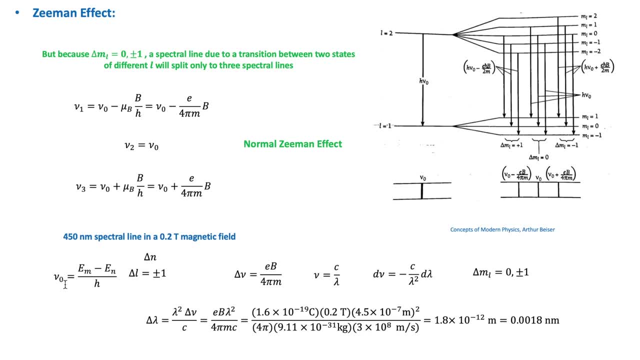 frequency of that photon or radiation is mu naught equal to em minus en over h. okay, and for this transition. so delta n, which is the difference between m and n, is not restricted, as we mentioned in the previous slide, for any transition. but delta l is restricted and it has to be either plus or minus one, because this is the selection rule for